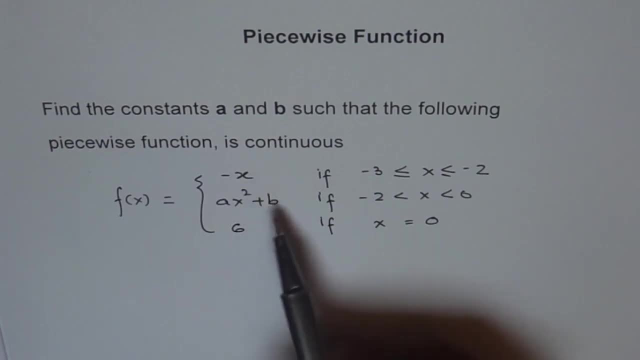 So the only possibility where they could be discontinuous is the points where they are joined together. right Now. here, what we should do is we should actually plug in the value of minus 2 here, because it's valid for minus 2.. And this function is not valid for minus 2,. 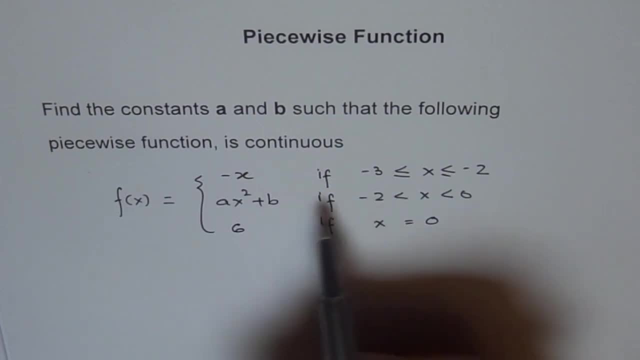 but when it is greater than minus 2, then it should kind of start from that value, correct? So in a way, at minus 2, this function should give us the same value as the previous one. Then they will be continuous at that point. 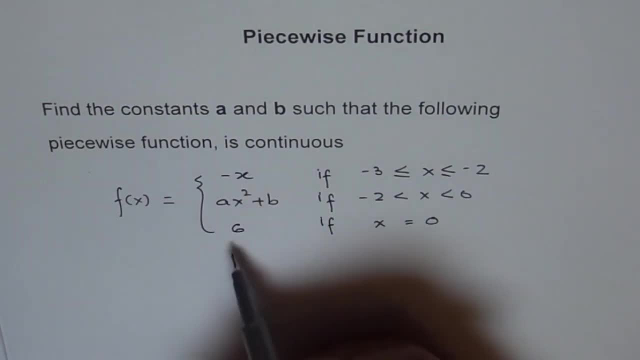 Now, in this particular case, at x equals to 0, both functions should have the same value. So that is the strategy which we are going to follow: And And then solve for the variables a and b. Since there are two variables to be found, we need two different equations to solve for them. 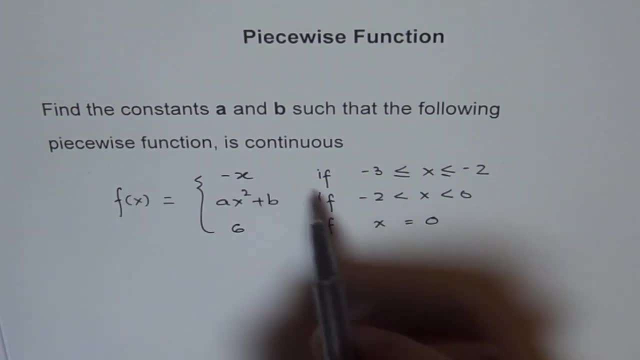 So we should get two equations, one from equating x equals to minus 2, and the other by equating x equals to 0. So let's start with x equals to minus 2.. So, at x equals to minus 2,, what we have is that these two functions should yield the same value. 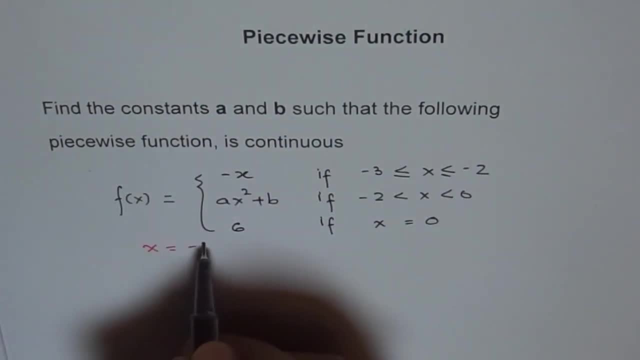 So let's see: At x equals to minus 2, what are we expecting? We are expecting that this value of minus x should be equal to this value, a x squared plus b, right? So if we plug in minus 2 here, we get minus of minus 2 equals to a times minus 2 squared plus b. 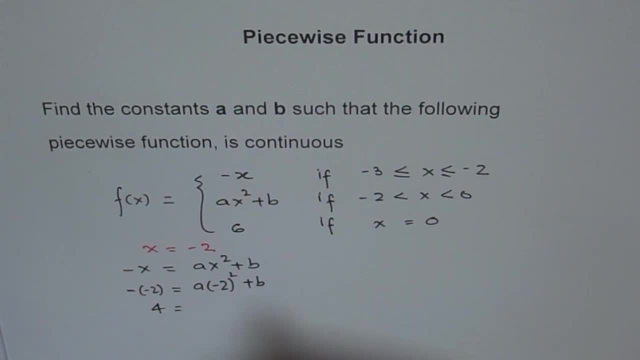 Now solving this, we get 4 equals to. This is 4a Plus b, right. So 4a plus b is 4 from this equation, right? The other condition which we have is: at: x equals to 0.. 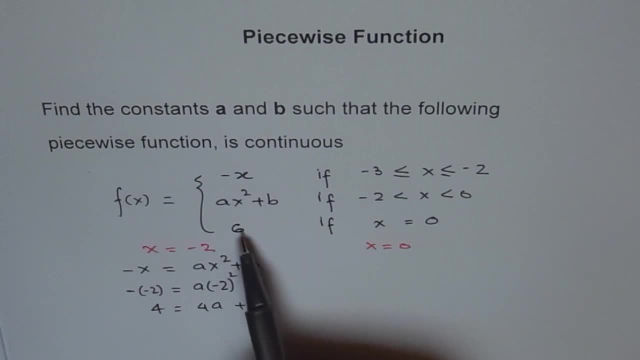 So at x equals to 0,. what do we expect? We expect that these two values should be same. Now, at x equals to 0, we have 6 here, right? So 6 should be equal to a times 0 squared plus b. is that okay? 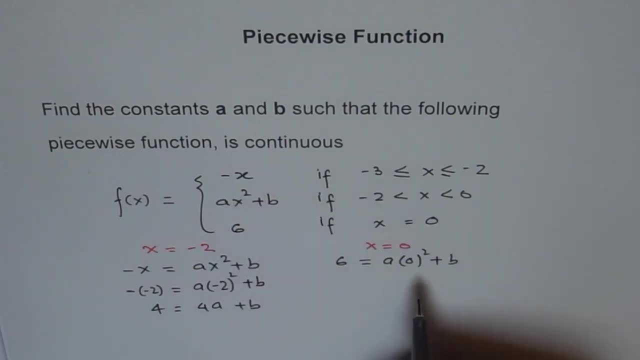 At x equals to 0, I just straight away plugged in the value 0. This gives me 6 equals to b. So that gives me the value of b. So that is the value of b, for which this kind of function will be continuous with this piece. 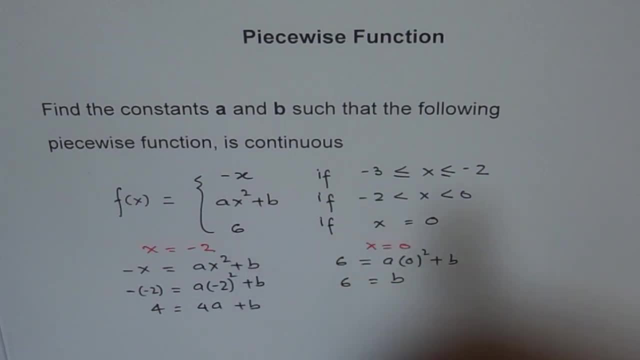 Okay, Now see, if you plug in 0 here, then b is 6, then you get a value 6, correct. Now in the first equation which is here Here, we have 4 equals to 4a plus b. 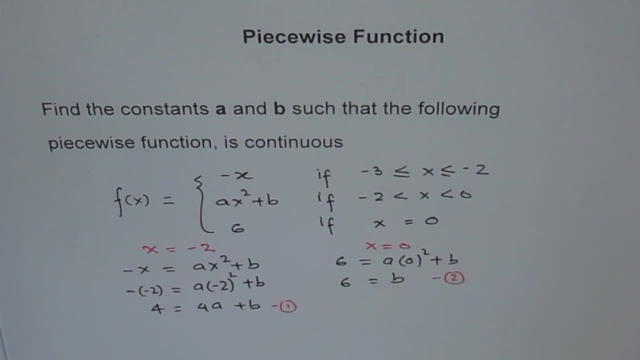 And from the second equation we get b equals to 6.. So we can substitute b from here in the first equation and then solve for a, correct. So once we do that now we'll substitute these two and then say 4 equals to 4a plus. 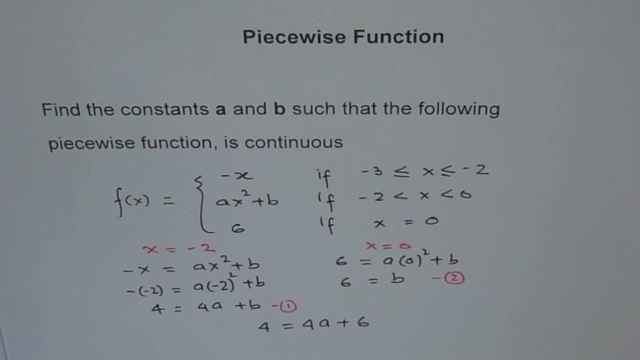 Instead of b, I'm writing 6, right, And then I'm going to solve for a, So it is 4.. Minus 6 equals to 4a, right, Which gives us a. equals to: This is minus 2 divided by 4.. 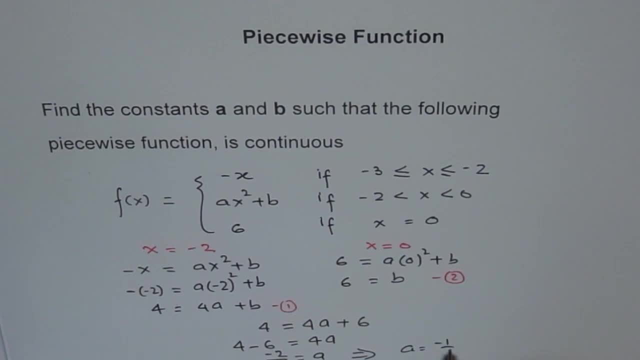 So we give a equals to minus half, correct? So that's how we solve. So this is from. We got this value of b from here, right, And this equation from here, And we equated the two to solve for a correct. 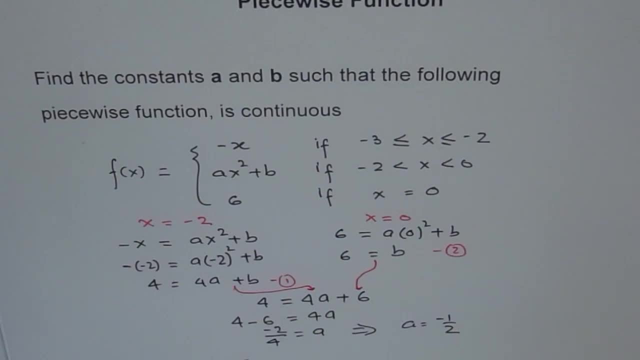 Therefore, the solution before us is that a should be equals to minus half and b should be equals to 6, correct? So I can write down the answer here: that a equals to minus half and b equals to 6, correct? So that is the solution. 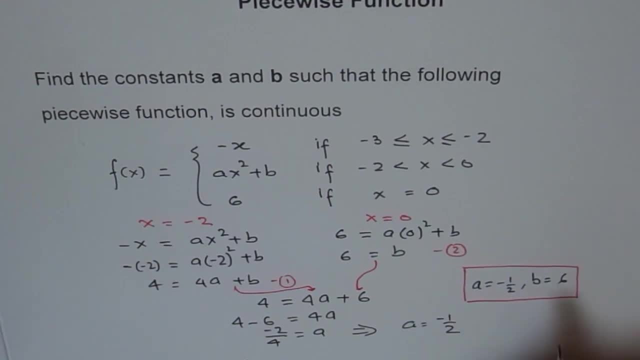 And for these values, this function should be continuous, correct. So that is how we need to solve piecewise functions for continuity, And it is not necessary that always we'll get some values for which the function is continuous. Sometimes it may be just impossible to make them continuous, okay. Thank you.